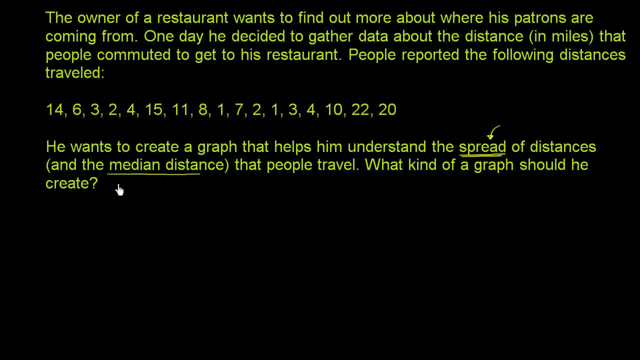 So what graph captures both of that information? Well, a box and whisker plot. So let's actually try to draw a box and whisker plot, And to do that, we need to come up with the median, and we'll also see the median of the two halves of the data. 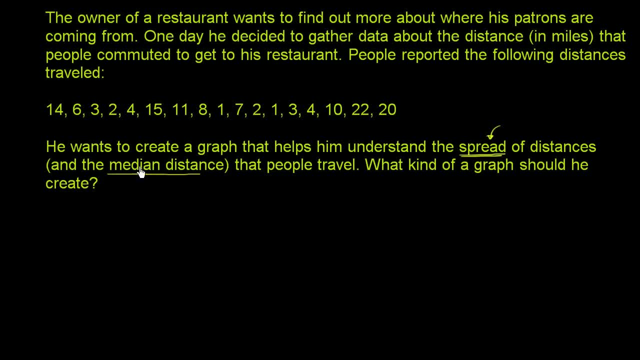 as well, And whenever we're trying to take the median of something, it's really helpful to order our data. So let's start off by attempting to order our data. So what is the smallest number here? Well, let's see, There's one- 2,, so let me mark it off. 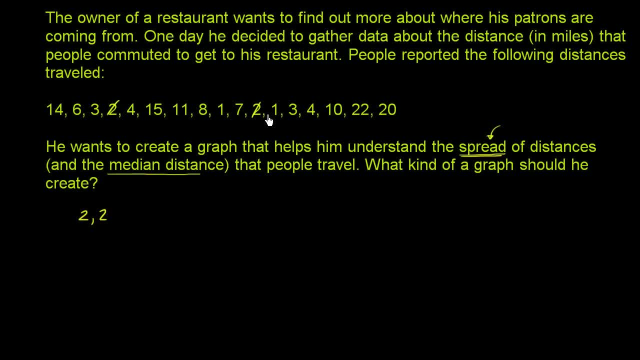 And then we have another 2, so we've got all the 2's, And then we have this, Then we have this 3.. Then we have this 3.. I think we got all the 3's. Then we have that 4.. 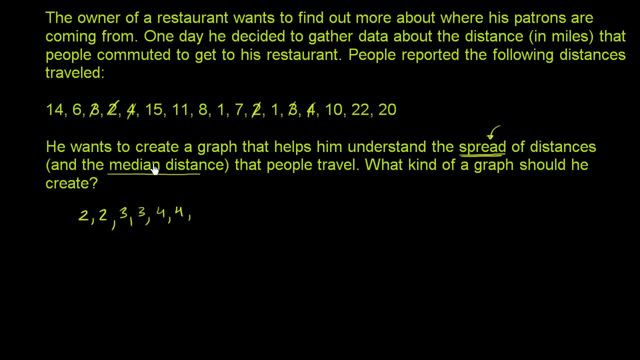 Then we have this 4.. Do we have any 5's? No, Do we have any 6's? Yep, we have that 6. And that looks like the only 6.. Any 7's? Yep? we have this 7 right over here. 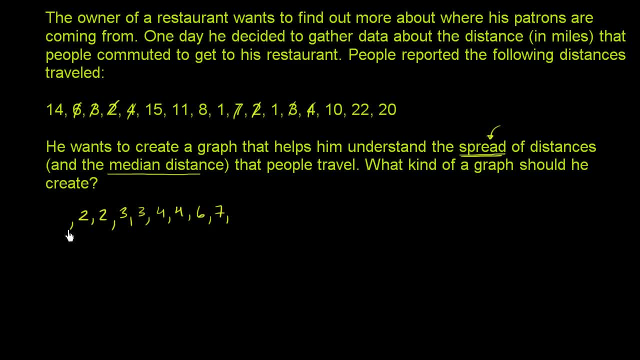 And I just realized that I missed this 1, so let me put the 1 at the beginning of our set. So I got that 1. 1 right over there. Actually, there's 2 1's. I missed both of them. 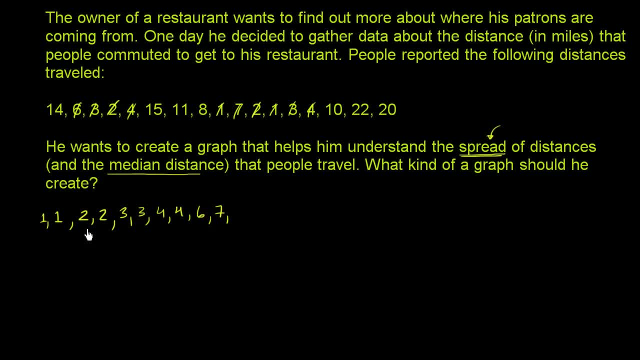 So both of those 1's are right over there. So I have 1's, 2's, 3's, 4's, no 5's. This is one 6. There was one 7. There's one 8 right over here. 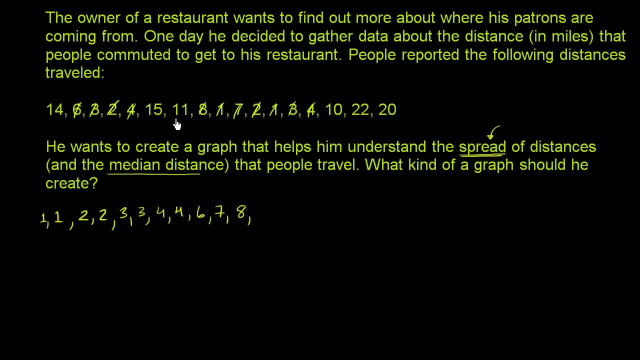 One, 8.. And then let's see any 9's, No 9's, Any 10's- Yep, there's a 10.. Any 11's- We have an 11 right over there- Any 12's. 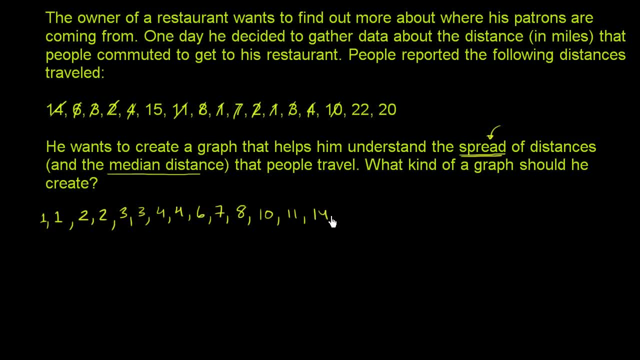 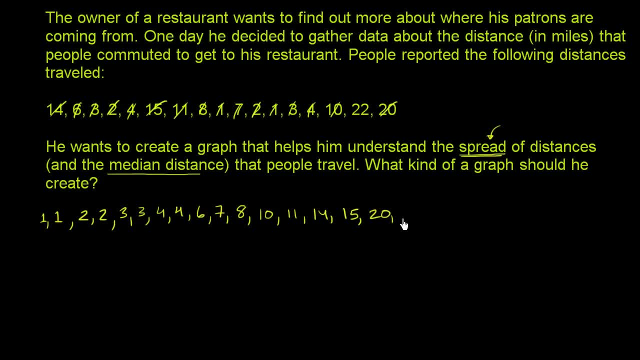 Then we have a 20.. And then a 22.. So we've ordered all our data. Now it should be relatively straightforward to find the middle of our data, the median. So how many data points do we have? 1,, 2,, 3,, 4,, 5,, 6,, 7,, 8,, 9,, 10,, 11,, 12,, 13,, 14,, 15,, 16,, 17.. 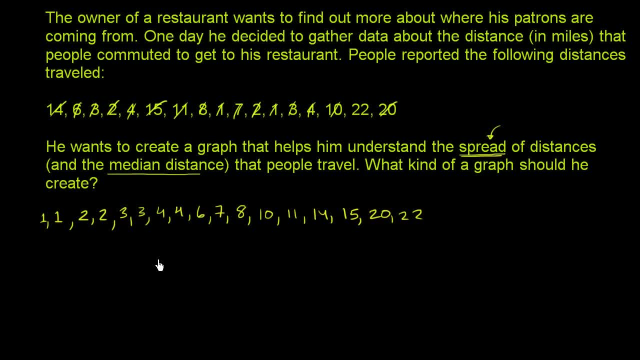 So the middle number is going to be a number that has 8 numbers larger than it and 8 numbers smaller than it. So let's think about it: 1, 2, 3, 4, 5, 6,, 7,, 8.. 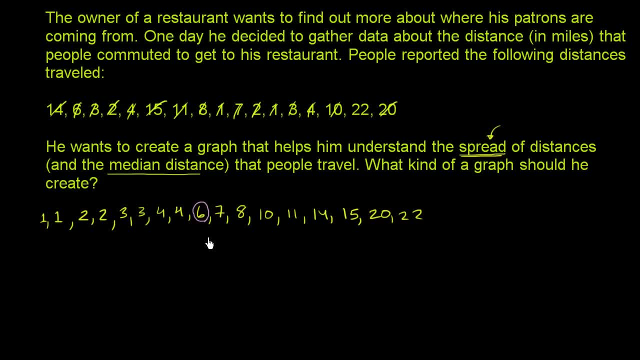 So the number 6 here is larger than 8 of the values And if I did the calculations right, it should be smaller than 8 of the values 1,, 2,, 3,, 4,, 5,, 6,, 7, 8.. 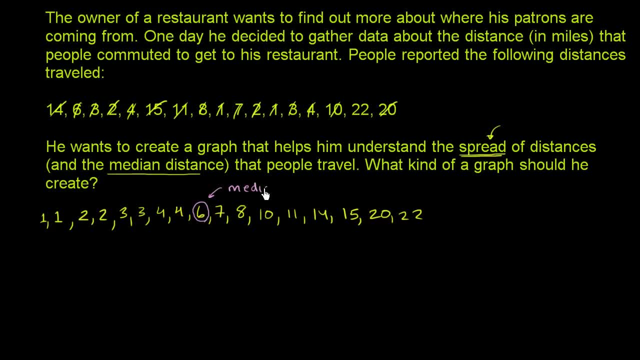 So it is indeed the median. Now, when we take a box and whisker, when we're trying to construct a box and whisker, plot, the convention is OK, we have our median And it's essentially dividing our data into two sets. 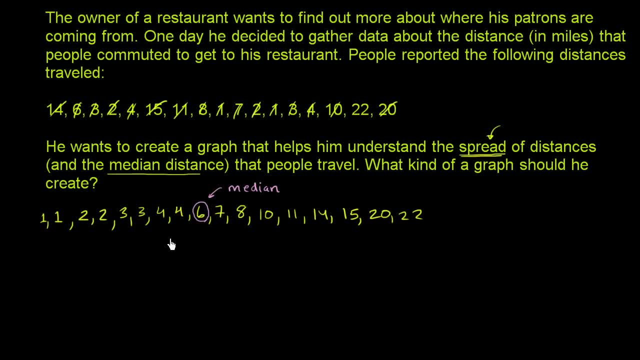 Now let's take the median of each of those sets, And the convention is to take our median out and have the sets that are left over. Sometimes people leave it in, But the standard convention take this median out and now look separately at this set. 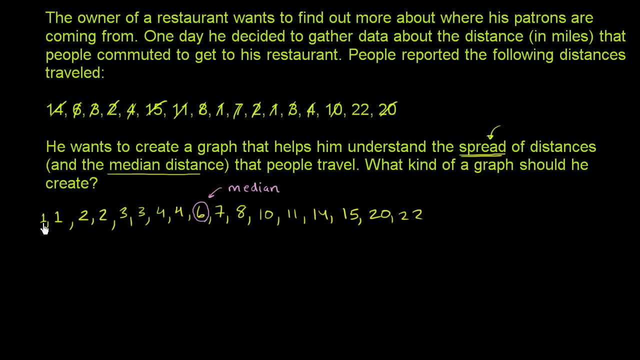 and look separately at this set. So if we look at this first, the bottom half of our numbers, essentially what's the median of these numbers? Well, we have 1,, 2,, 3,, 4,, 5,, 6,, 7, 8 data points. 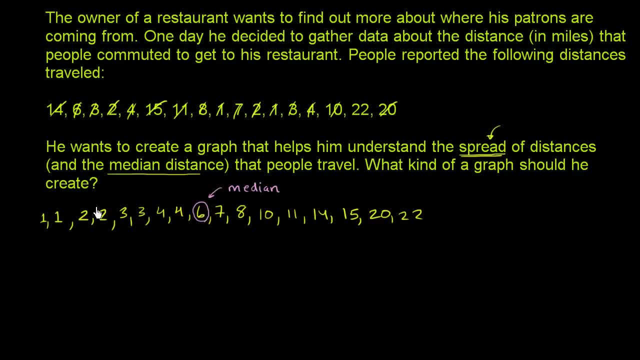 So we're actually going to have two middle numbers. So the two middle numbers are this 2 and this 3.. Three numbers less than these two, three numbers greater than it. And so when we're looking for a median and you have two middle numbers, we 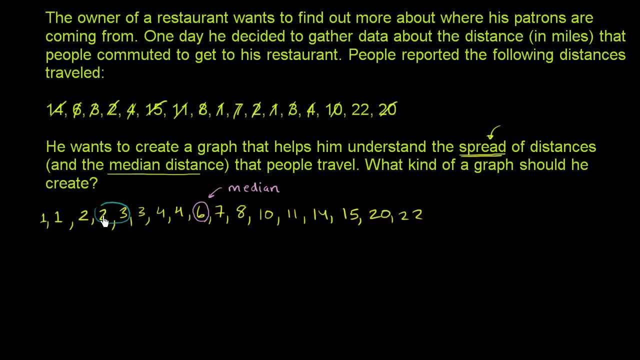 take the mean of these two numbers. So halfway in between 2 and 3 is 2.5.. Or you could say: 2 plus 3 is 5, divided by 2 is 2.5. So here we have a median of this bottom half of 2.5. 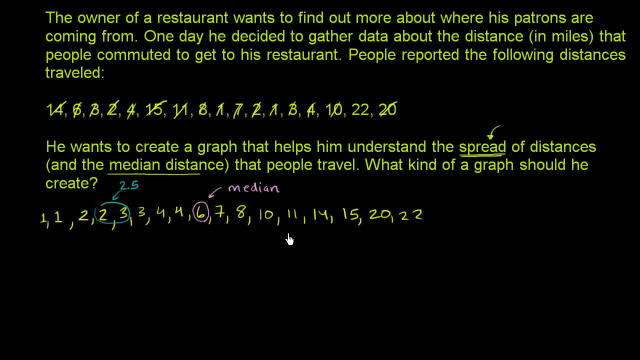 And then the middle of the top half. once again we have eight data points. So our middle two numbers are going to be this 11 and this 14.. And so, if we want to take the mean of these two numbers, 11 plus 14 is 25.. 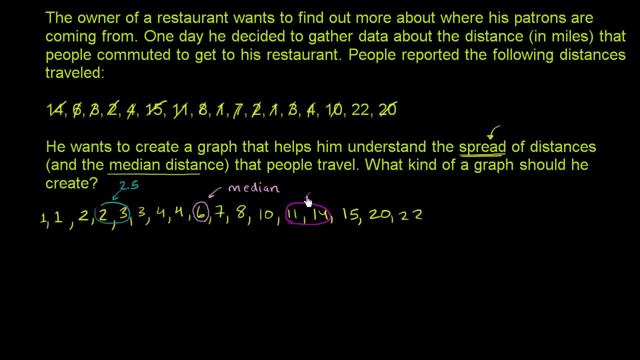 Halfway in between the two is 12.5.. So 12.5 is exactly halfway between 11 and 14.. And now we've figured out all of the information we need to actually plot or actually create, or actually draw our box and whisker plot. 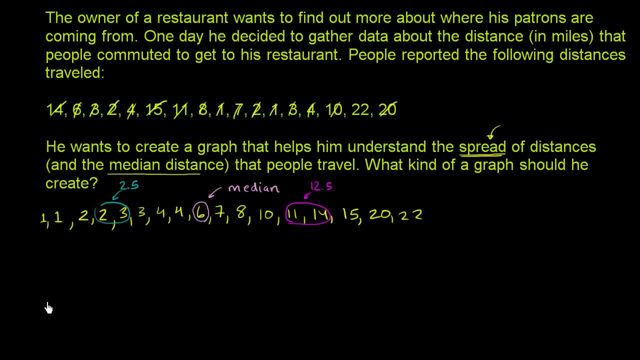 So let me draw a number line. Let me draw a number line. So my best attempt at a number line. So that's my number line, And let's say that this right over here is 0.. I need to make sure I get all the way up to 22 or beyond 22.. 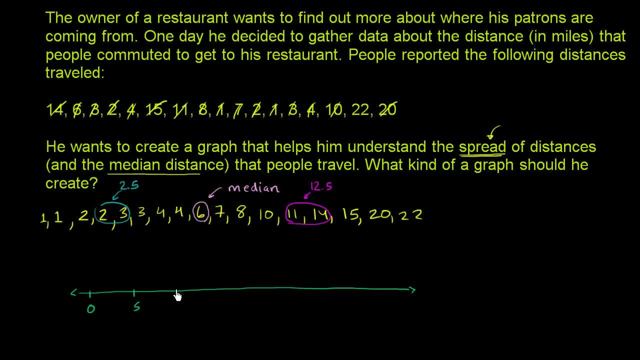 So let's say that's 0.. Let's say this is 5.. This is 10.. That could be 15.. And that could be 20.. This could be 25. And we could keep going: 30. It could be maybe 35.. 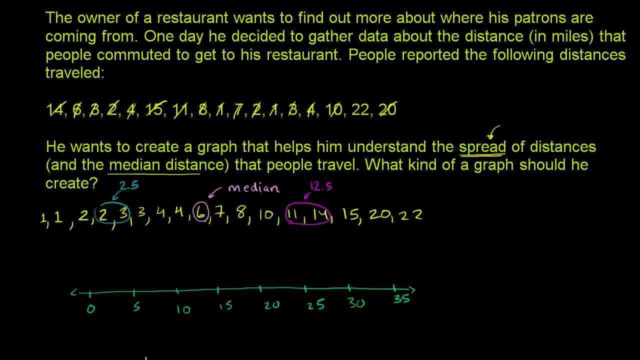 So the first thing we might want to think about- there's several ways to draw it- We want to think about the box, part of the box, and whisker essentially represents the middle half of our data, So it's essentially trying to represent this data right. 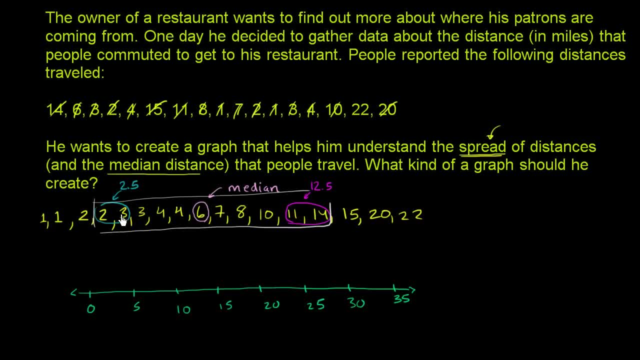 over here, So the data between the medians of the two halves. So this is a part that we would attempt to represent with the box. So we would start right over here At this: lower this 2.5,. this is essentially. 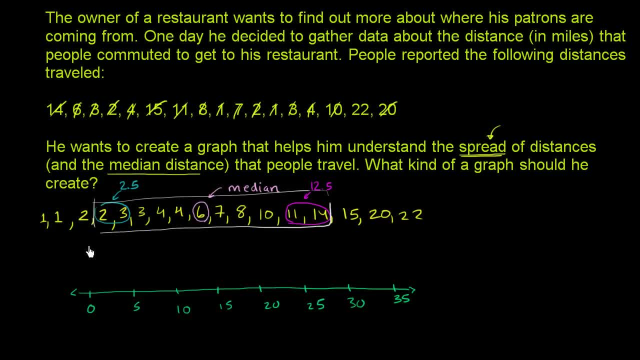 separating the first quartile from the second quartile, the first quarter of our numbers from the second quarter of our numbers. So let's put it right over here. So this is 2.5.. 2.5 is halfway between 0 and 5.. 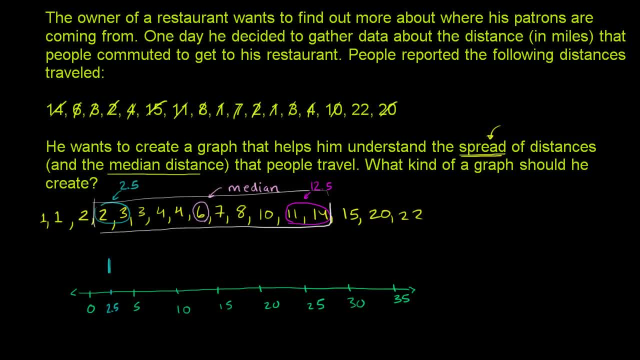 So that's 2.5.. And then up here we have 12.5. And 12.5 is right over. let's see, this is 10.. So this right over here would be 10.5.. This halfway between- well, halfway between- 10 and 15. 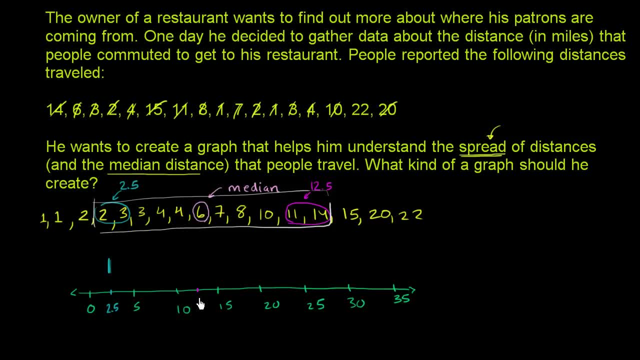 is 12.5.. So let me do this. So this is 12.5, right over here 12.5.. So that separates the third quartile from the fourth quartile, And then our box is everything in between. So this is literally the middle half of our numbers. 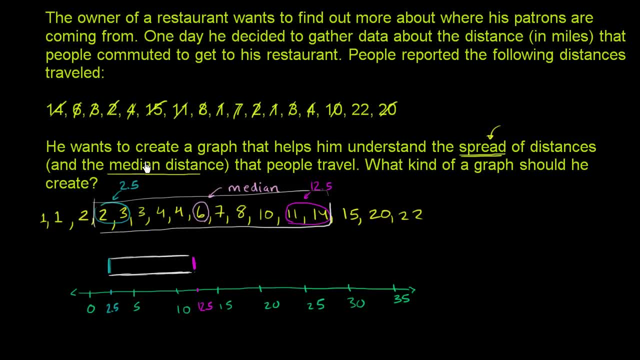 And we'd want to show where the actual median is, And that was actually one of the things that we wanted to be able to think about in our original, when the owner of the restaurant wanted to think about how far people are traveling from. So the median is 6.. 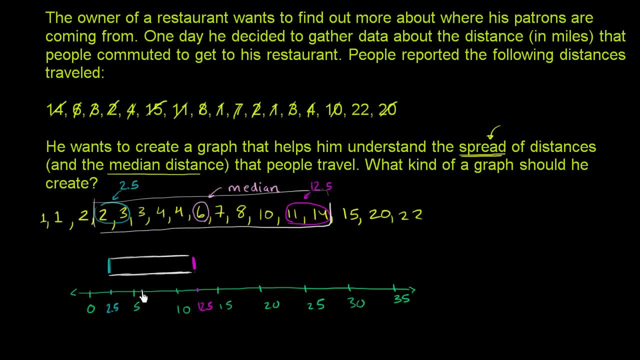 So we can plot it right over here. So this right over here looks this is about 6.. So that is, let me do that same pink color. So this right over here is 6.. And then the whiskers of the box and whisker plot. 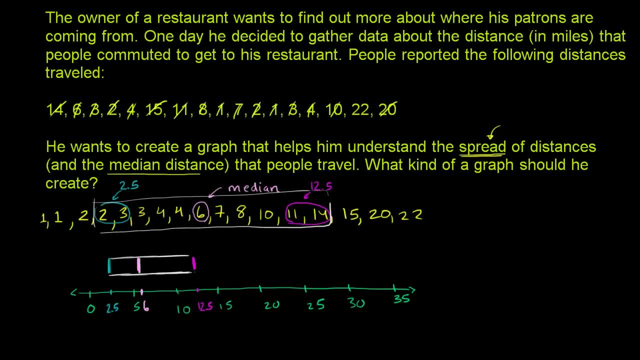 essentially show us the range of our data, And so let me do that. I could do this in a different color that I haven't used yet. I'll do this in orange. So, essentially, if we want to see, look the numbers go all the way up to 22.. 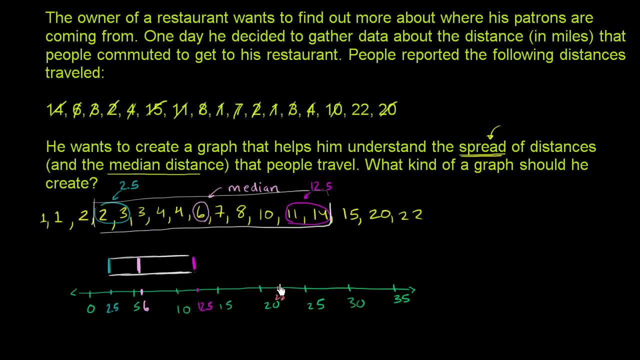 So they go all the way up to 22.. So let's say that this is 22 right over here. Our numbers go all the way up to 22. Our numbers go all the way up to 22. And they go as low as 1.. 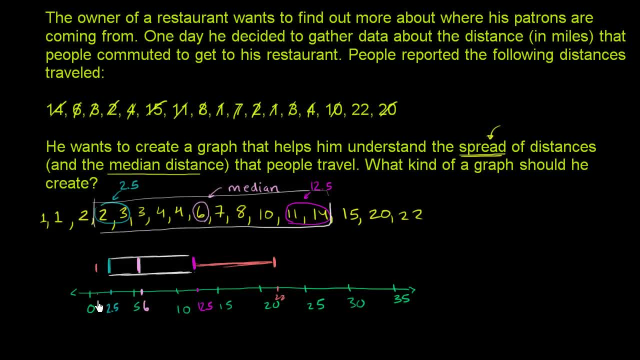 So they go. 1 is right about here. They go as low. let me label that. so that's 1.. And they go as low as 1.. So there you have it. We have our box and whisker plot. 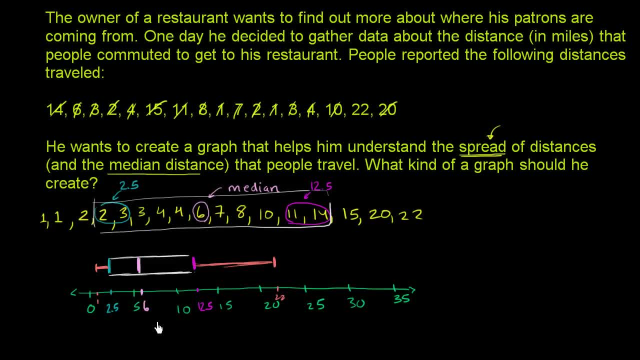 And you can see if you have a plot like this. just visually, you can immediately see. OK, what is the median? It's the middle of the box. Essentially, It shows you the middle half, So it shows you how far they're spread. 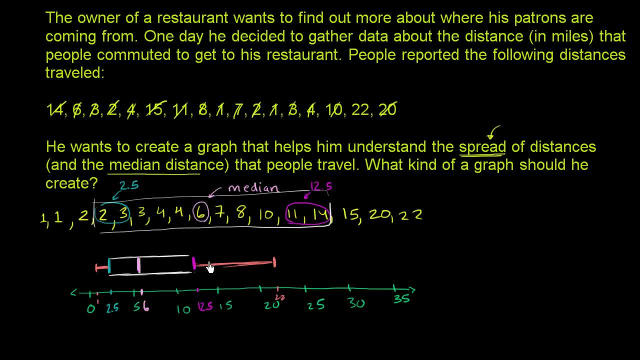 or kind of where the meat of the spread is, And then it shows, well beyond that we have, the range that goes well beyond that, or how far the total spread of our data is. So this gives a pretty good sense of both the median 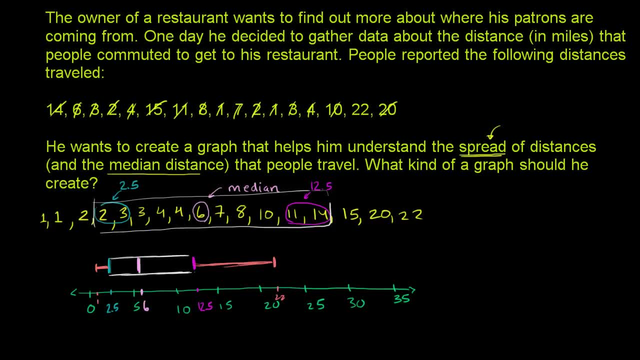 and the spread of our data.